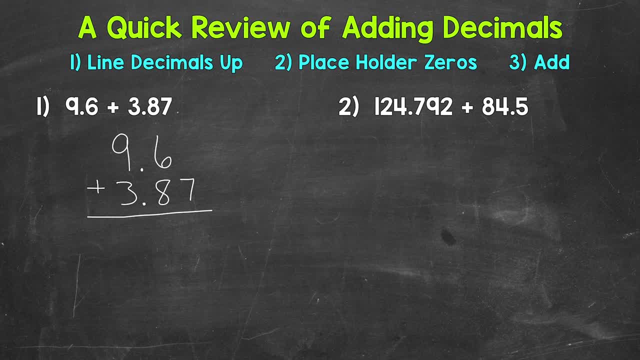 Remember, zeros to the right of a decimal do not change the value of that decimal. So we're going to be working with an equivalent decimal. We're not changing the value of the problem at all. So we're able to use placeholder zeros to the right of a decimal. So let's put a zero here in the hundredths place. And now both of our numbers go to the hundredths. And we're able to add. So we'll start with the hundredths. 0 plus 7 is 7. 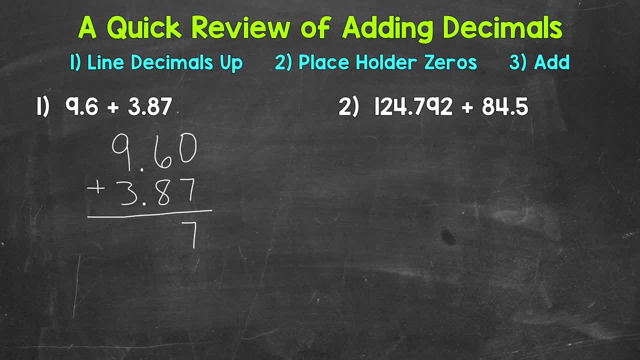 Then we'll move to the tenths. 6 plus 8 is 14. So we carry our 1. Now our decimal goes straight down into our answer. It's lined up throughout the entire problem. Now we'll move to the ones place where we have 1 plus 9 plus 3. 1 plus 9 is 10 plus 3 is 13. So we'll put our 3. And then our carried 1. And then our carried 1. 1 will be brought straight down. 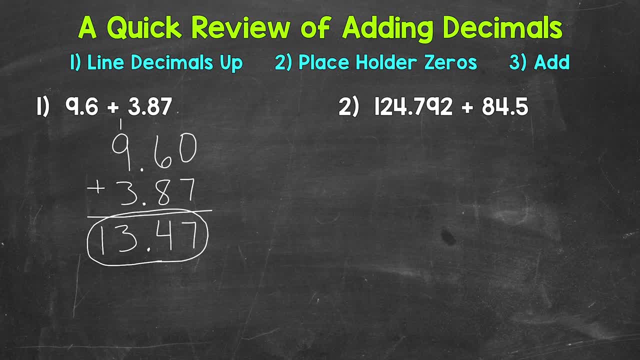 And we end up with 13 and 47 hundredths. 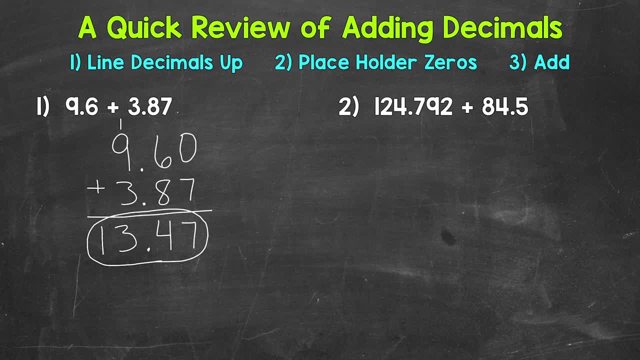 Let's move on to number 2 where we have 124 and 792 thousandths plus 84 and 5 tenths. So let's line our decimals up here. 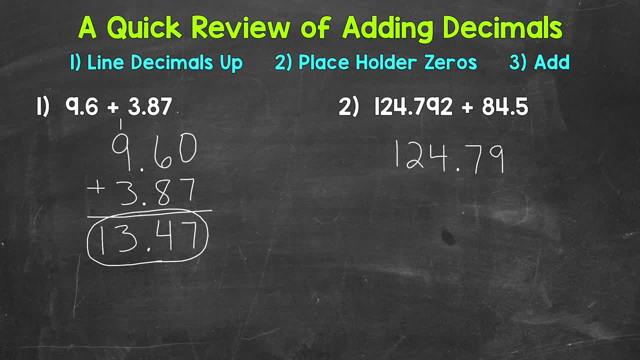 124 and 792 thousandths plus. 84 and 5 tenths. 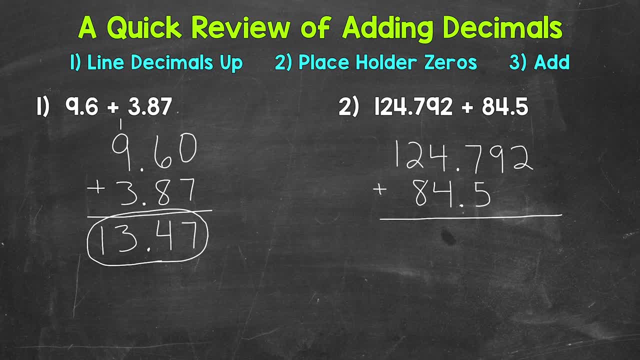 So let's use placeholder zeros to line this up a little better here. A zero in the hundredths. 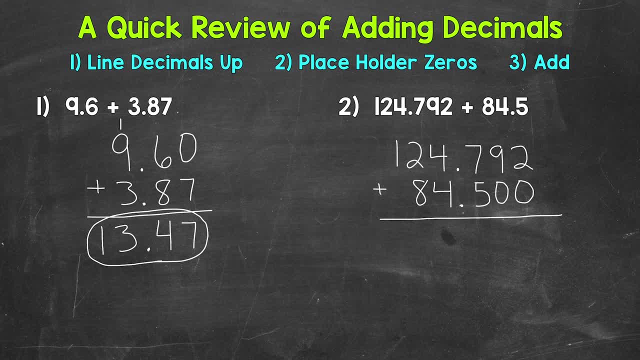 And then a zero in the thousandths. Again, zeros to the right of a decimal do not change the value of that decimal. 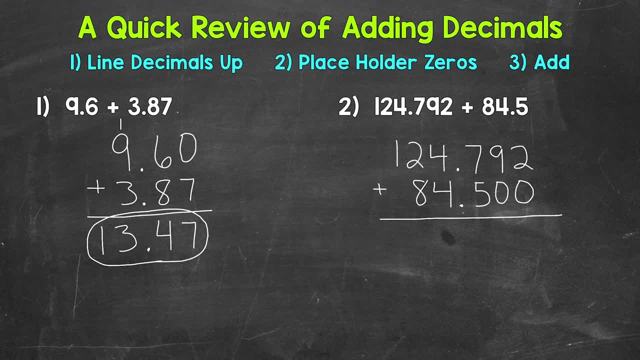 It's an equivalent decimal. So we're able to use those placeholder zeros. Now we can add. 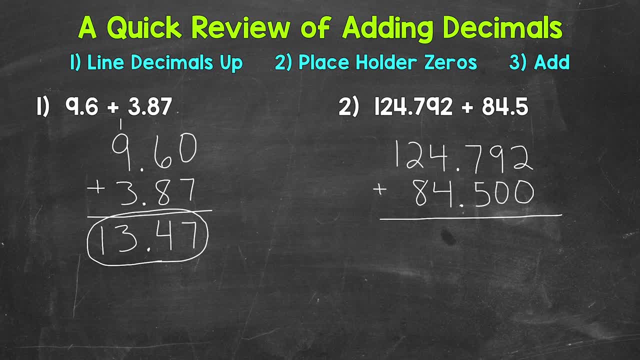 So we'll start with the thousandths place. 2 plus 0 is 2. The hundredths place. 9 plus 0 is 9. 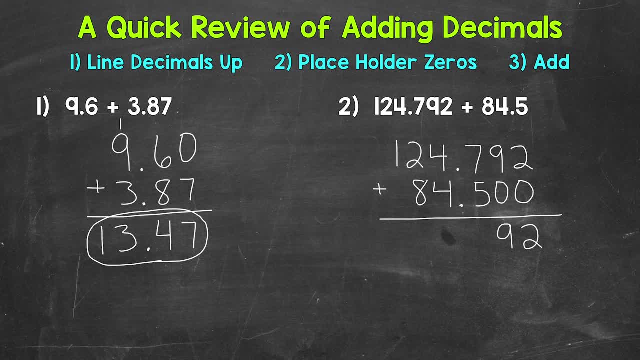 The tenths place. 7 plus 5 is 12. So we'll put our 2 and then carry the 1. We can bring our decimal straight down into the answer. Now we have the ones place. 1 plus 4 is 5 plus 4 is 9. The tens place. 2 plus 8 is 10. So we'll put our. 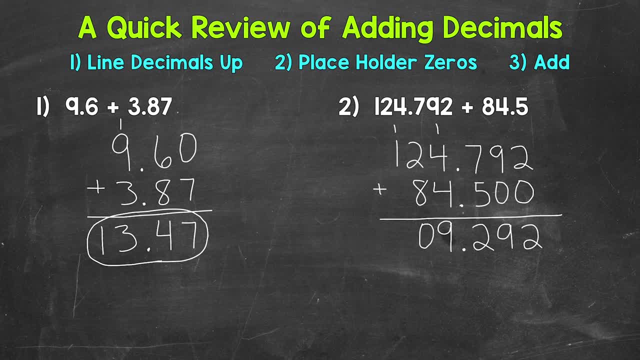 0 here, carry the 1, and then the hundredths place. 1 plus 1 is 2. So we end up with 209 and 292 thousandths. That's how we add decimals. Let's move on to subtraction. 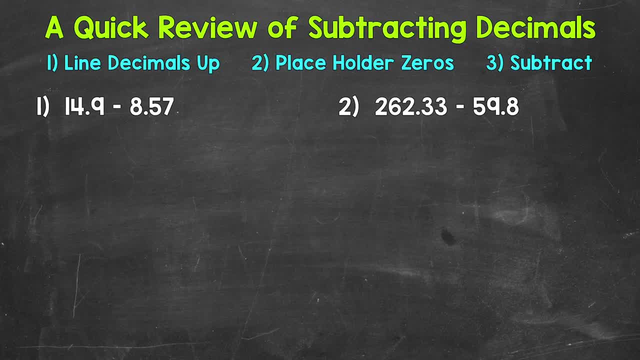 So here are our examples of subtracting decimals. Let's jump into number 1 where we have 14 and 9 tenths. Minus. 8 and 57 hundredths. 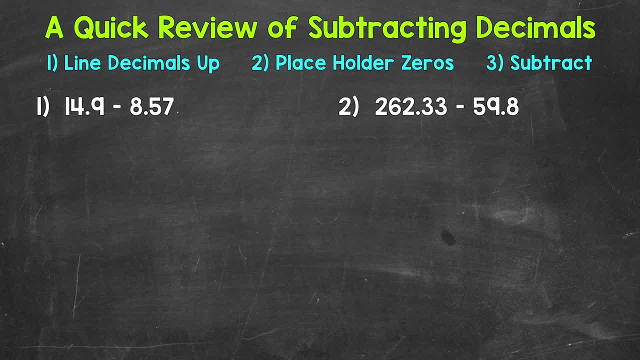 Now just like when we add decimals, when we subtract decimals, we need to line the decimals up. That's going to line up all of our places. 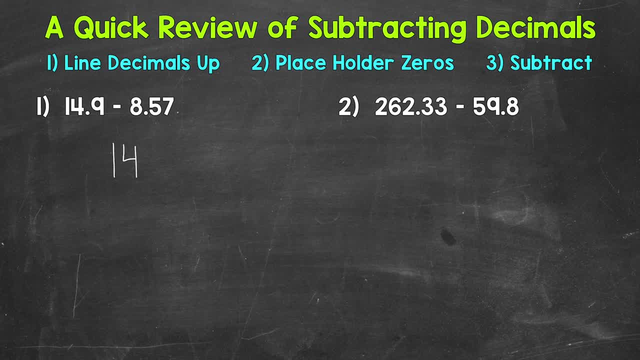 So let's rewrite this first problem vertically here, lining up the decimals. So 14 and 9 tenths minus 8 and 57 hundredths. 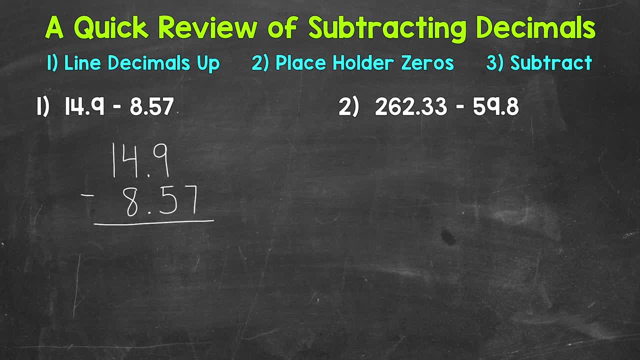 So the decimals are lined up. And that's going to line up all of our places. 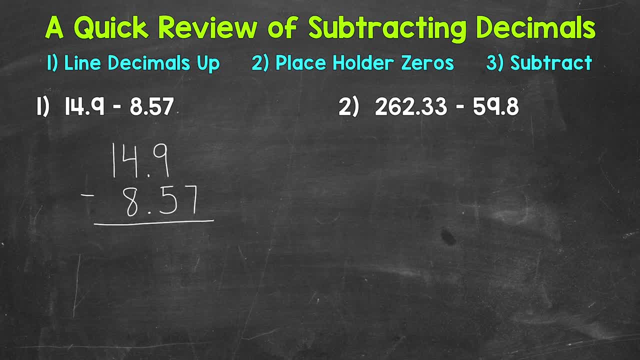 Now that problem looks a little offset because 14 and 9 tenths goes to the tenths place, and then 8 and 57 hundredths goes to the hundredths place. So just like when we add decimals, we can use placeholder zeros to have this look more lined up. So let's use a placeholder zero in the hundredths place here, and then both of our decimals go to the hundredths place. Remember, zero is to the right of a decimal. So that's going to line up all of our places. 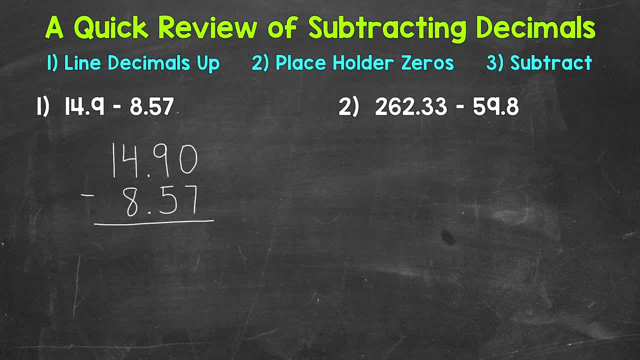 But the decimals do not change the value. That's an equivalent decimal, and does not change the value of the problem at all. 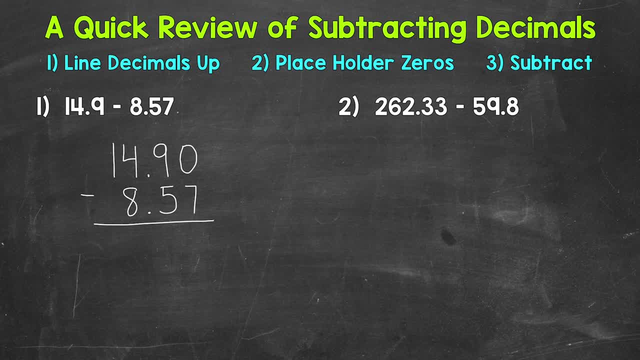 Now we're able to subtract. So we'll start with the hundredths place. We have zero minus seven, which we need to borrow. So let's borrow from the nine, that's an eight now. And we have ten minus seven, which is three. Then we move to the tenths place. Eight minus five. Three. 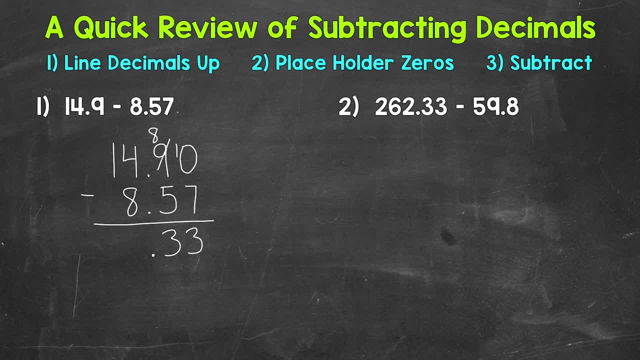 Three. Bring our decimals, two back. decimal straight down into the answer the decimal is lined up throughout the entire problem then we 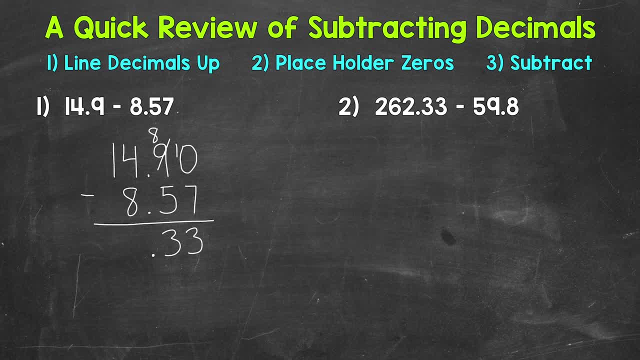 move to the ones place four minus eight we need to borrow from the tens place here so that's a zero and that's a 14. so 14 minus 8 is 6 and we are done 6 and 33 hundredths now i do want to mention 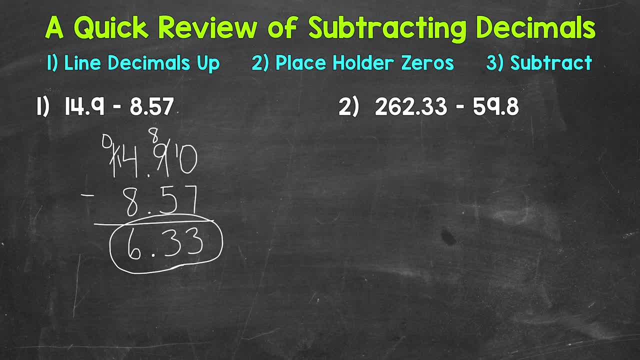 one more thing before moving on to number two and this is going to be a common mistake that you'll want to avoid and using placeholder zeros will actually help you avoid this mistake so let me rewrite the problem here real quick to the side so we have 14 and nine tenths minus 8 and 57 hundredths 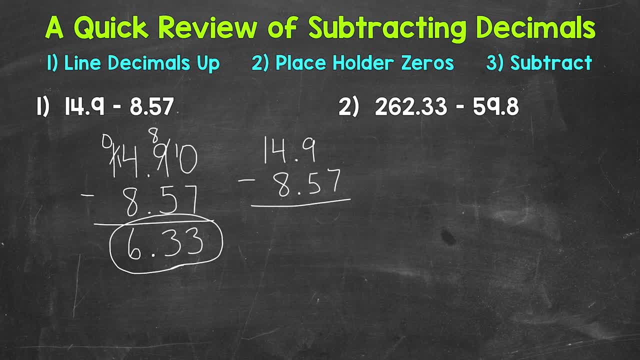 so dropping this seven so starting with the hundredths place and then just dropping this seven because there isn't anything above it is not correct. We actually have zero minus seven there so we needed to borrow and you can see we do not have a seven in the hundredths place in our final answer. So again avoid the mistake of just dropping that number because really we have 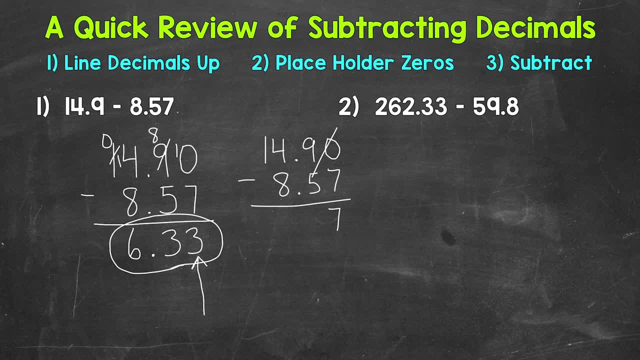 zero minus seven there and we need to borrow. So be careful of that. Let's move on to number two 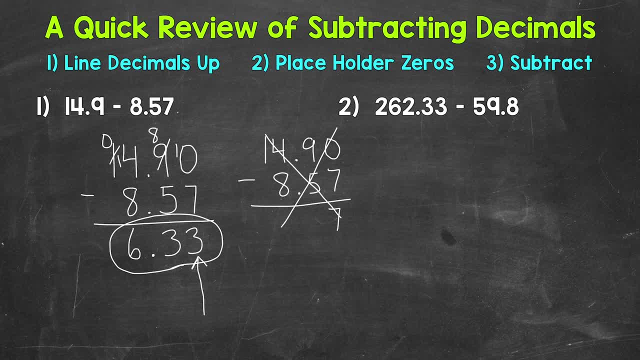 where we have 262 and 33 hundredths minus 59 and 8 tenths. So we will start by lining up our 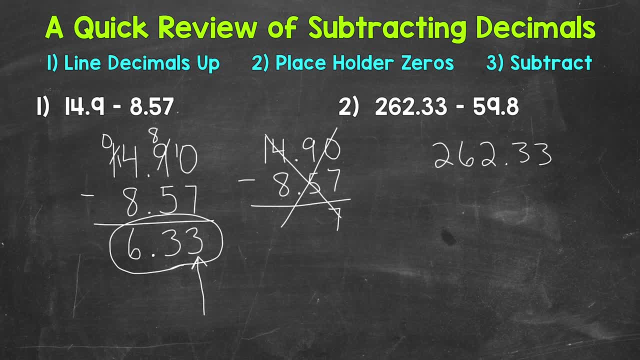 decimals here. So 262 and 33 hundredths minus 59 and 8 tenths. We can use a placeholder zero so 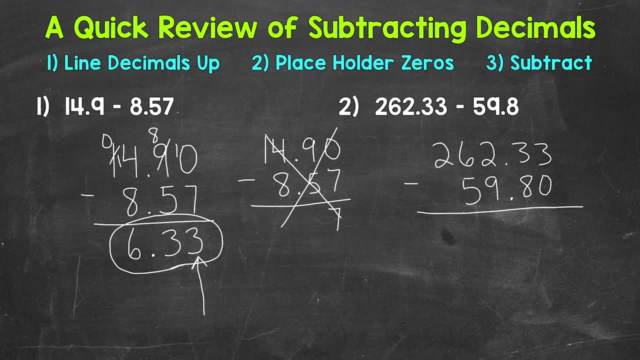 these both go to the hundredths and now we are able to subtract. So we'll start by lining up our decimals here. So 262 and 33 hundredths minus 59 and 8 tenths.